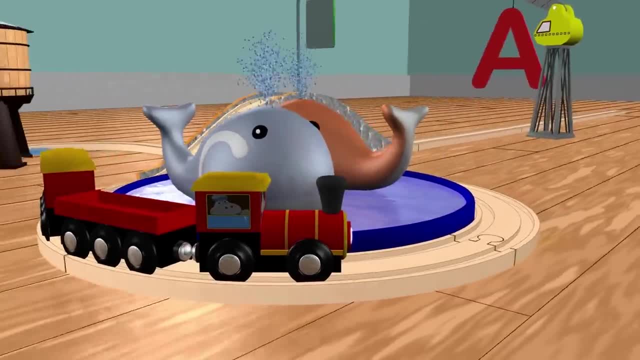 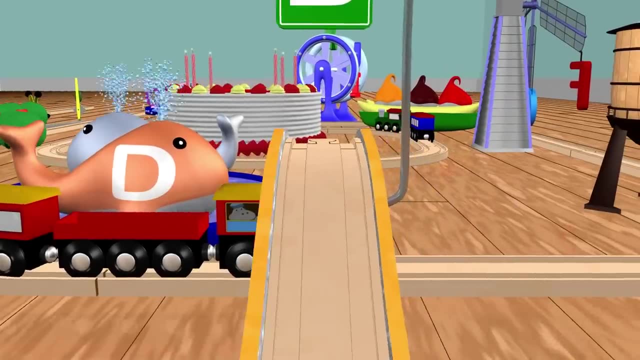 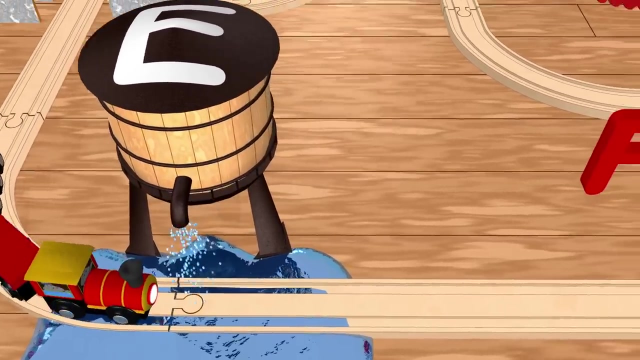 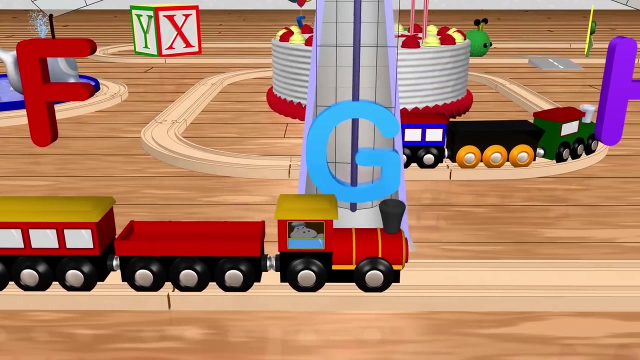 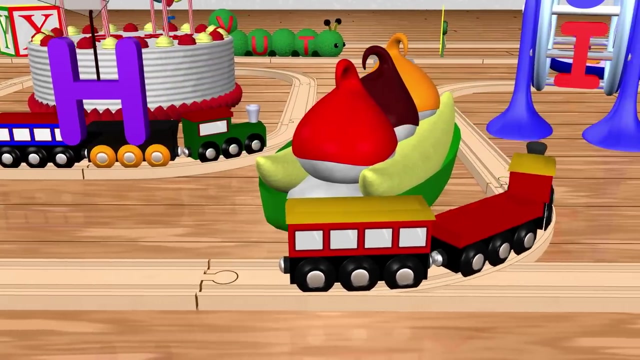 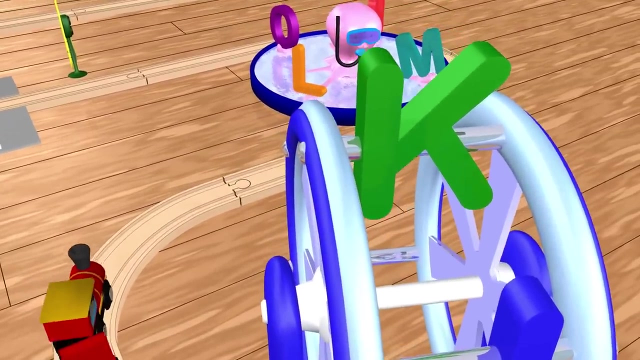 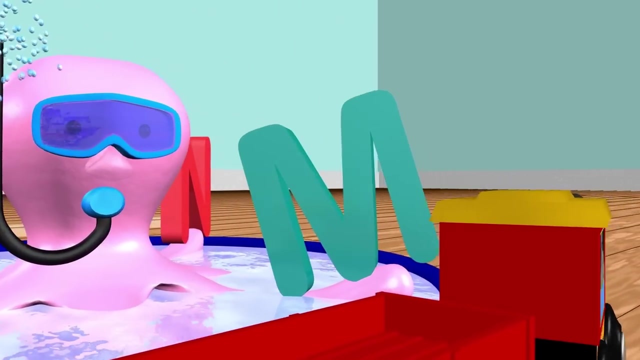 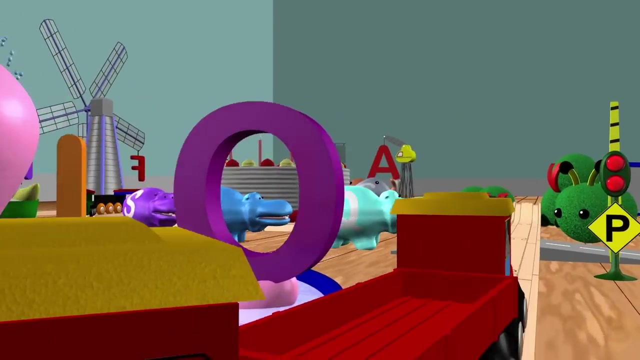 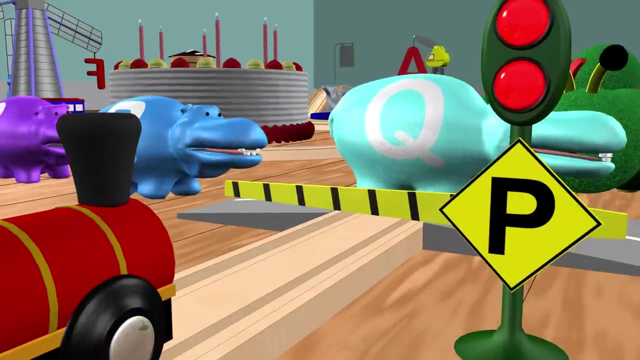 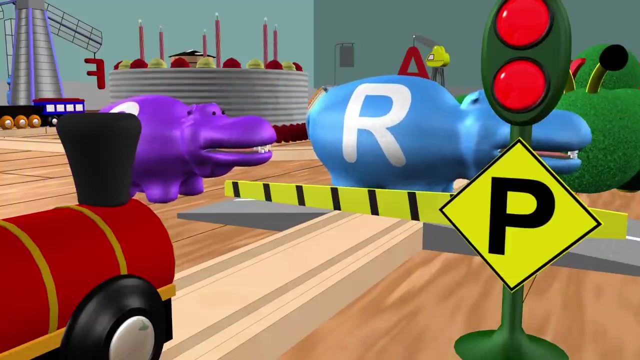 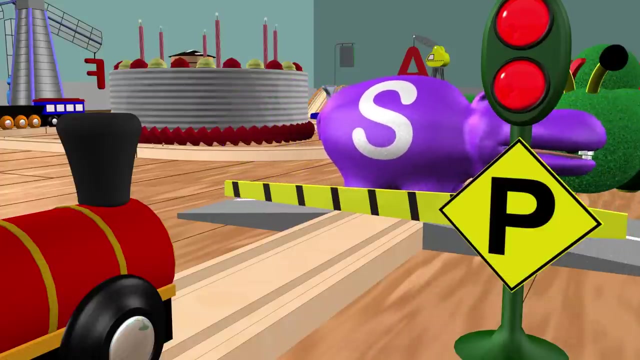 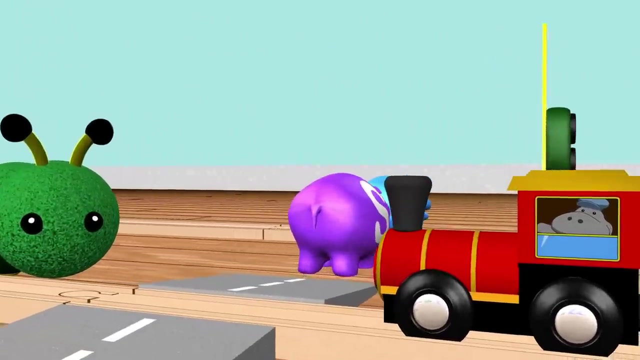 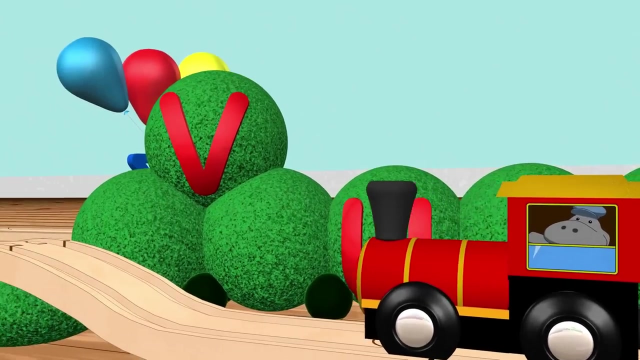 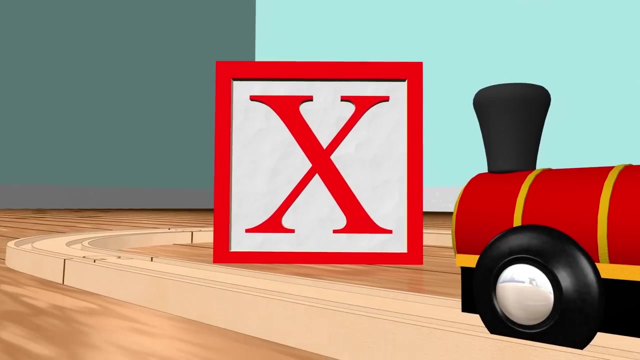 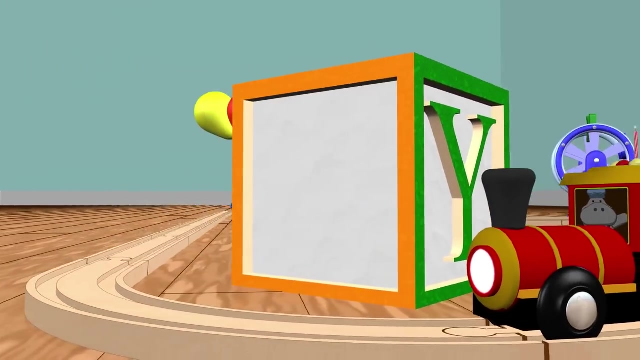 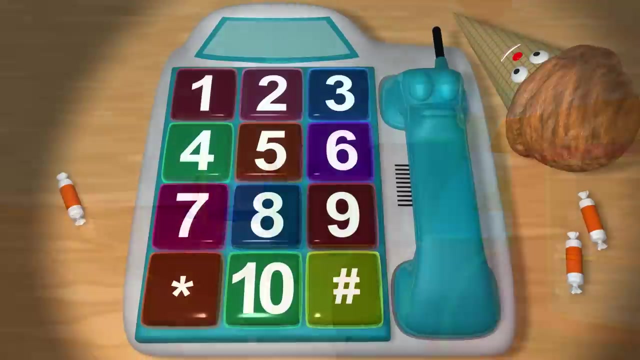 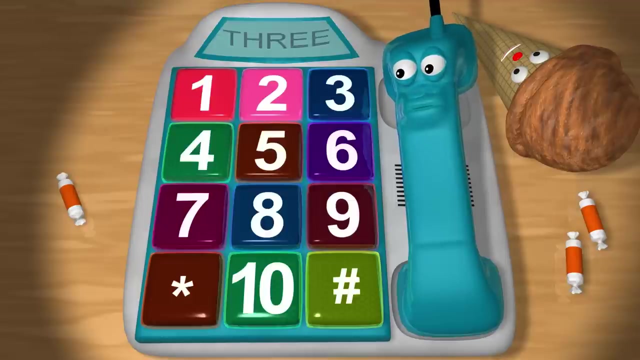 B, B, C, D, E, F, G, H, I, J, K, L, M, N, O, E, Q, R, S, T, U, V, W, X, Y, Z. Let's count: One, Two, Three, Four, Five, Six, Seven, Eight, Nine, Ten Again. One, Two, Three, Four, Five, Six, Seven. 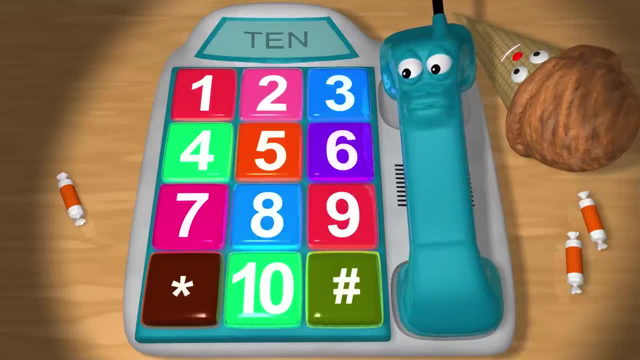 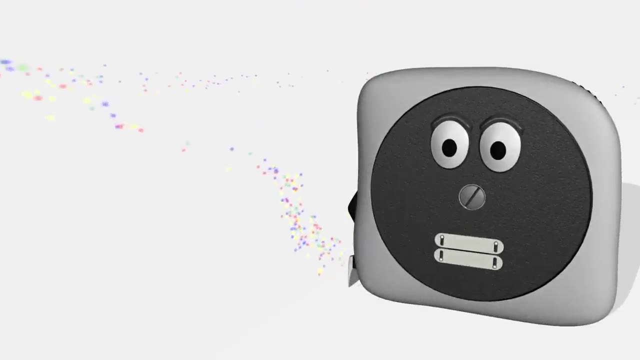 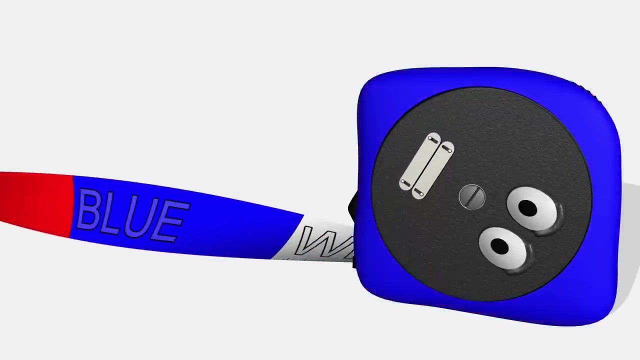 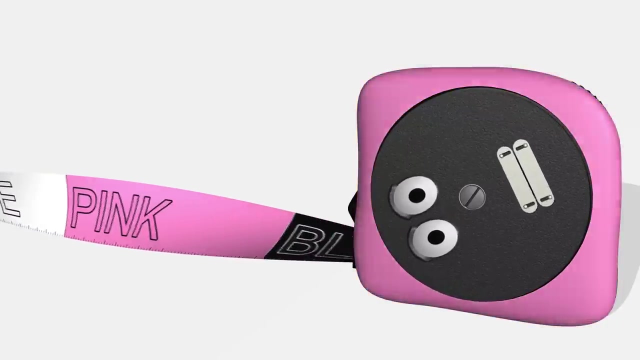 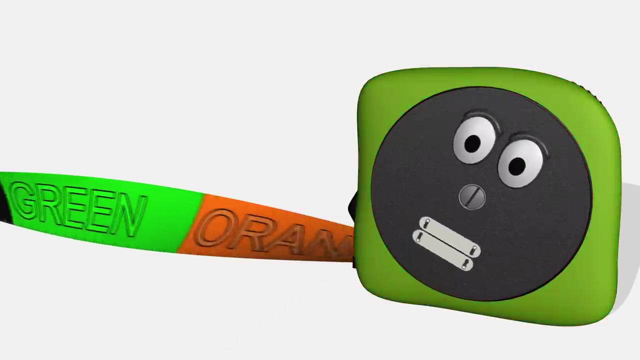 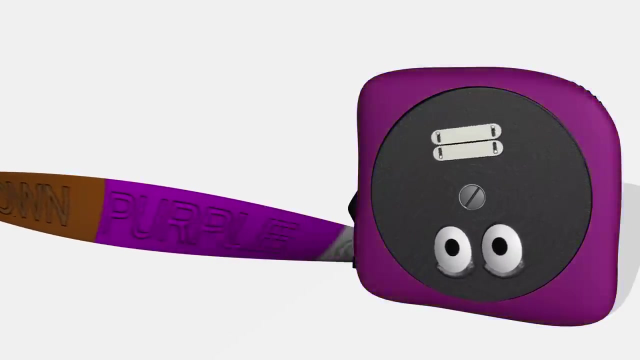 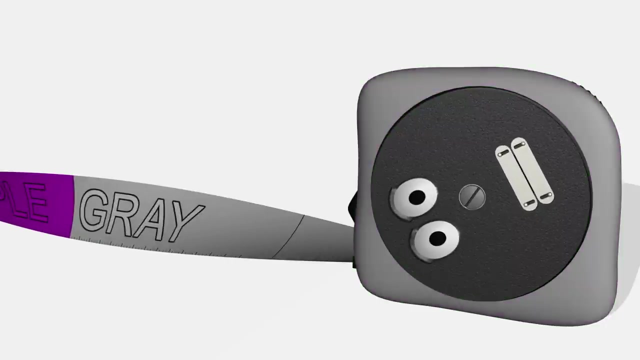 Eight Nine, Ten Ice cream. One, Two, Three, Four, Five, Six, Seven, Eight Nine, Ten. One, Two, Three, Four, Three, Two. One, Two, One, Two, Three, Four, Three. Two, One, Two, One, Two, Three, Three, Rock. One, Two, Three, Two, One, Two, Three, Four, Four. Three. One, Two, Three, Two, Four. 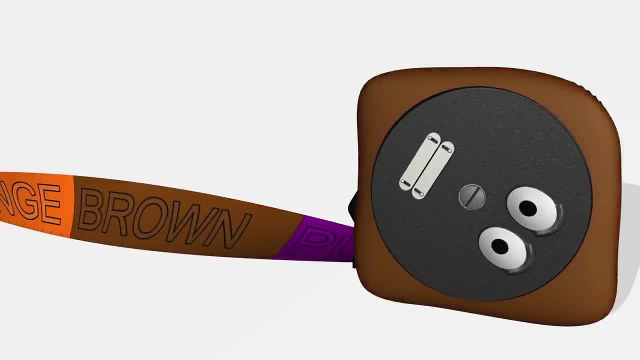 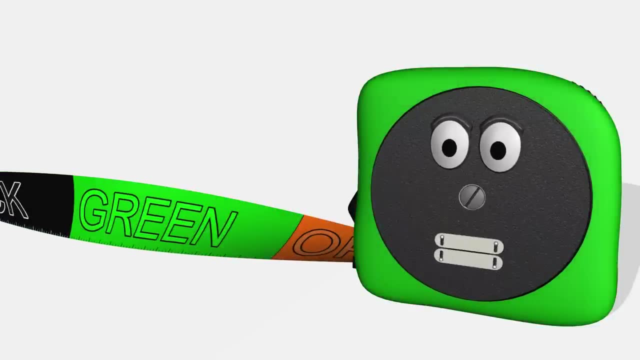 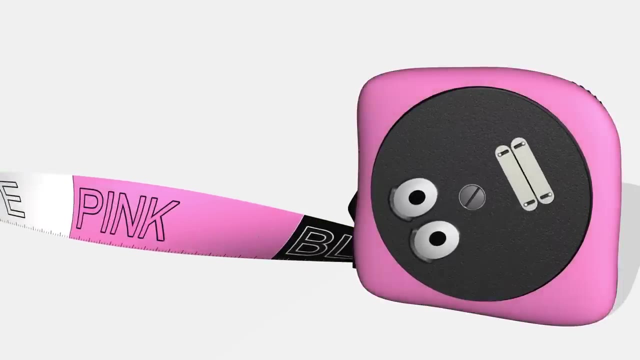 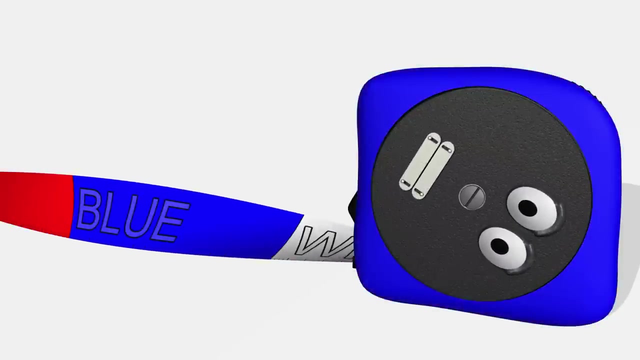 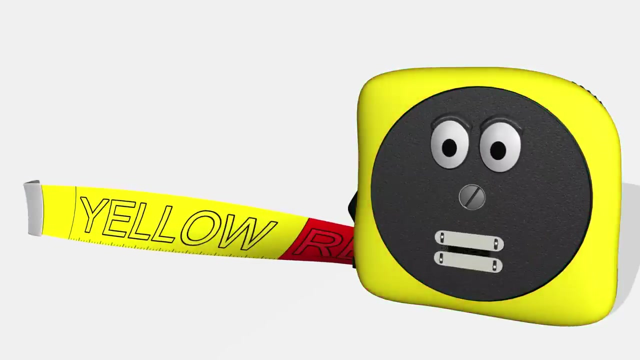 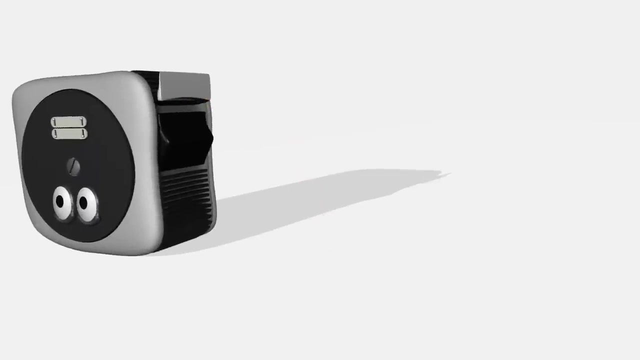 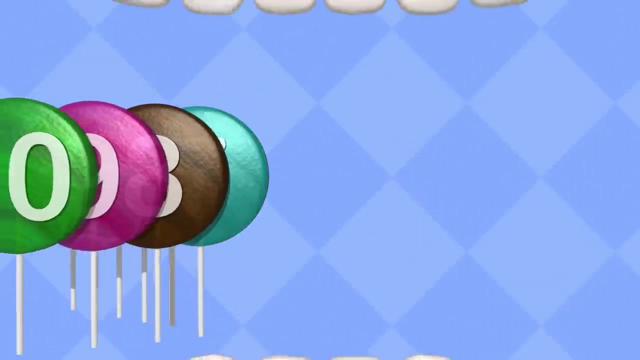 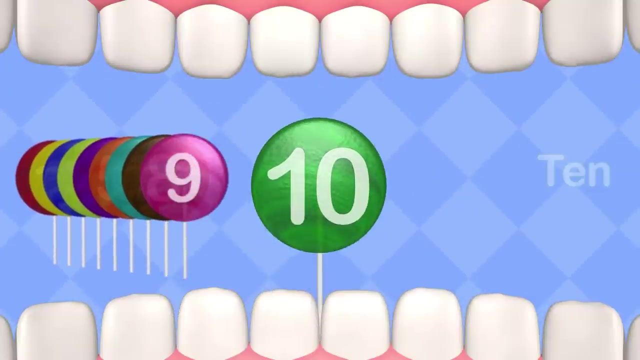 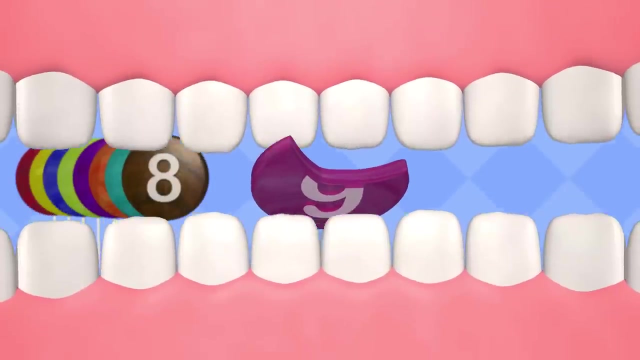 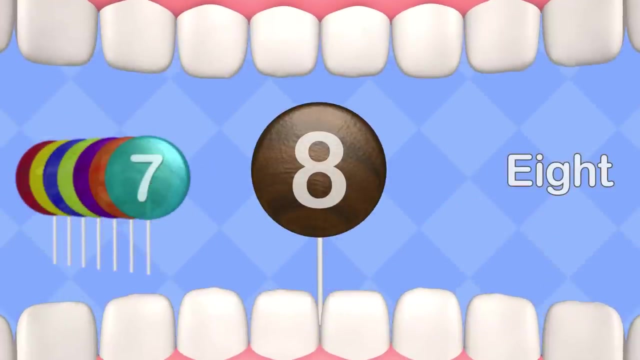 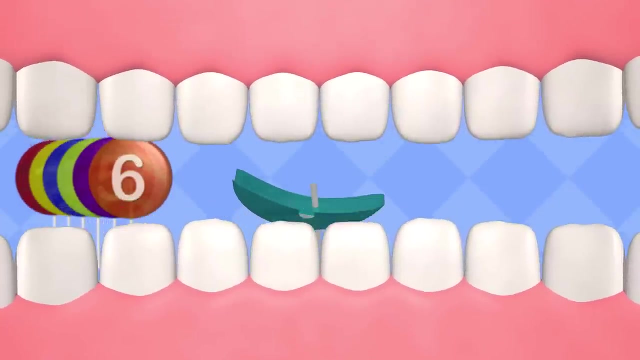 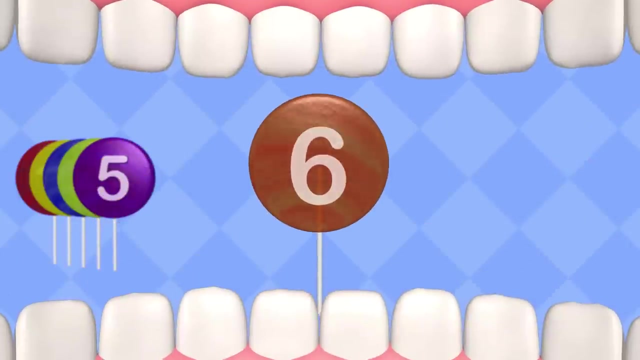 Three, Four, Five, Four, Seven, Seven exhibit rushed Rock. Why Black, Pink, White, Blue, Red, Yellow? Uh-oh, Let's count down from 10, 10, 9, 8, 7, 6, 7, 8, 8, 8, 9, 10, 10, 10. 12, 13, 14, 14, 15, 15, 16, 18, 19, 20, 21, 22, 23, 24, 25, 26, 27, 28, 29, 30, 31, 32, 32, 33, 34, 35. 36, 37, 38, 38, 39, 39, 40, 41, 42, 42, 43, 44, 44, 45, 46, 47, 47, 48, 49, 49, 50, 51, 52, 53, 53, 54. 53, 54, 53, 54, 55, 56, 56, 57, 57, 58, 58, 58, 58, 59, 59, 51, 53, 53, 53, 54, 55, 56, 57, 58, 59, 53. 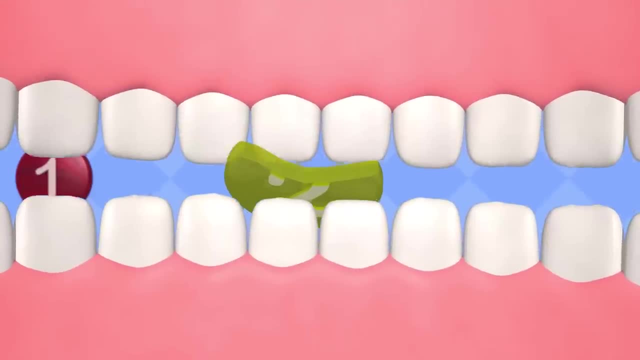 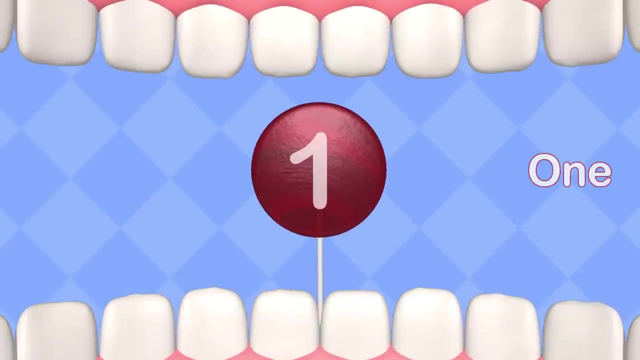 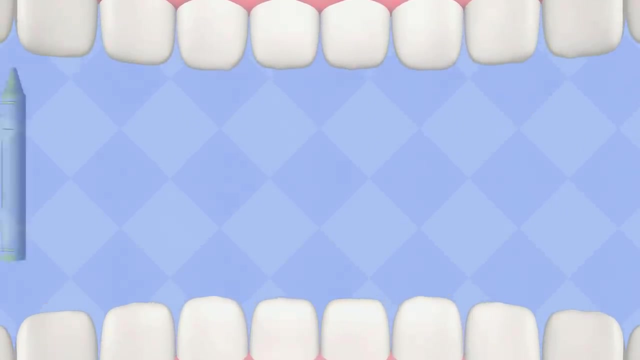 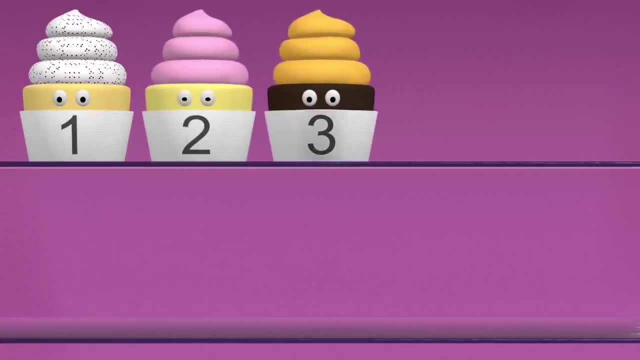 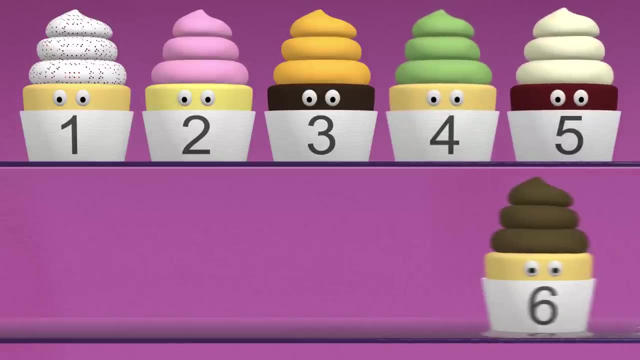 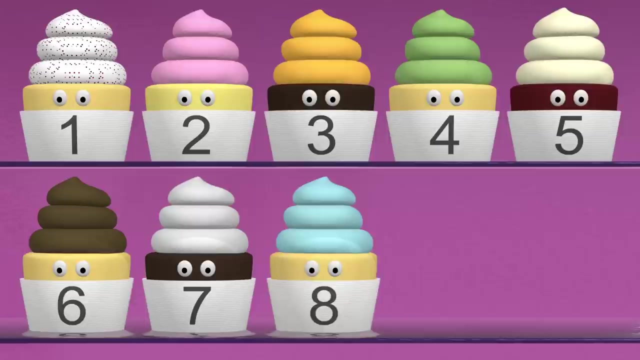 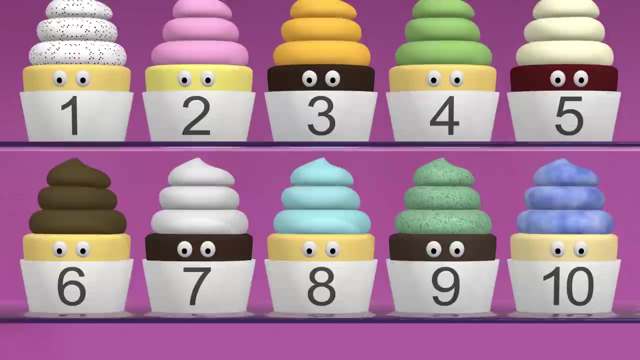 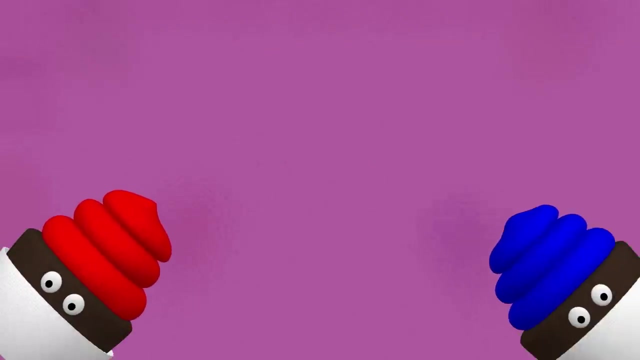 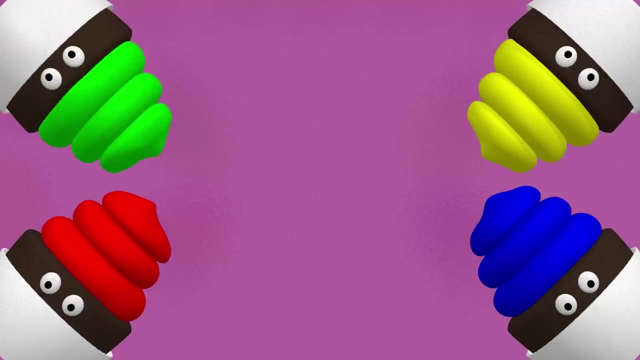 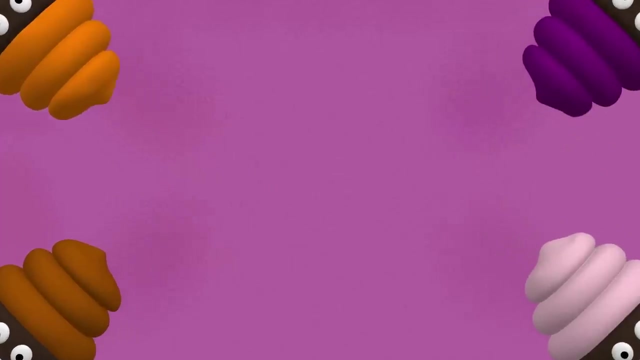 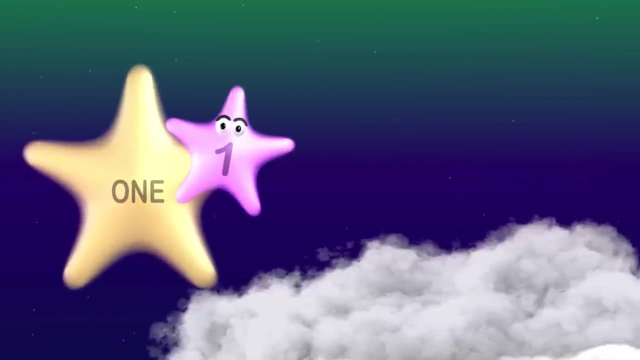 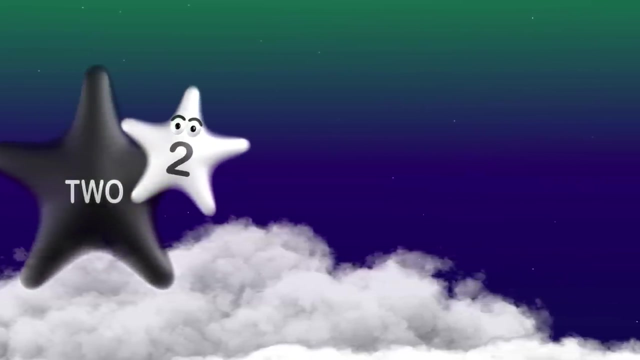 2, 3, 4, 5, 6, 7, 8, 9, 10 Red, Blue, White, Blue, Red, Blue, Red, Blue, Yellow, Green, Green, Brown, Brown, Pink, Orange, Orange, Purple. Let's count, Let's count One One, Two, Two, Three, Two, Three, Two. 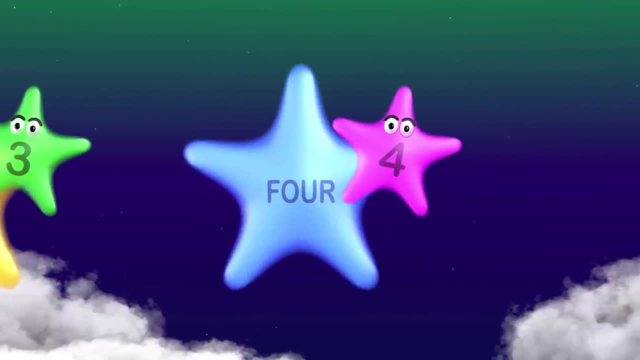 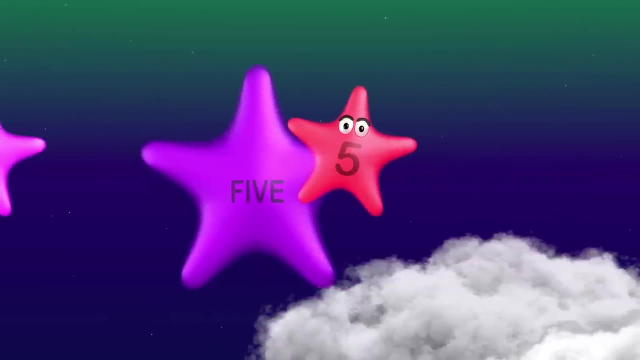 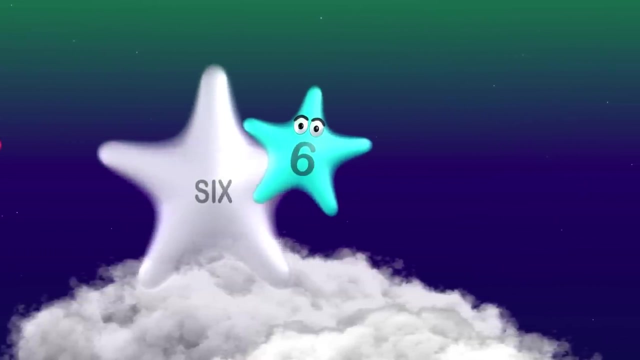 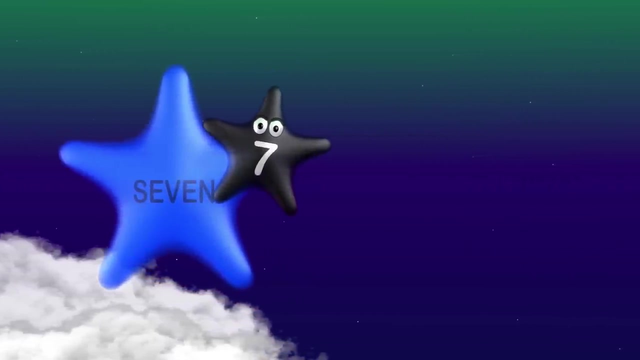 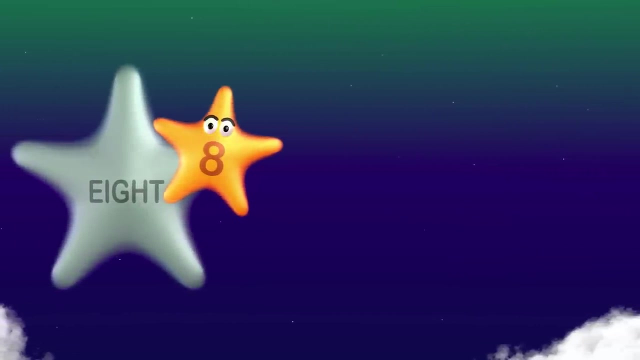 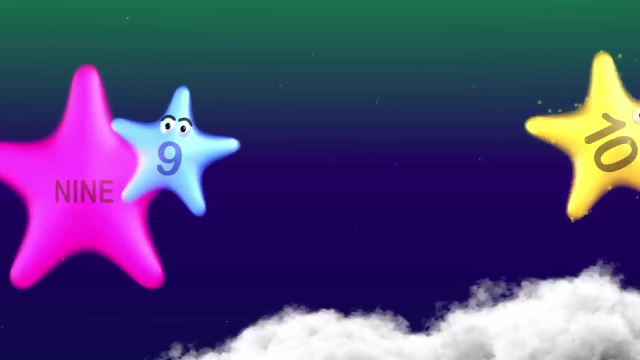 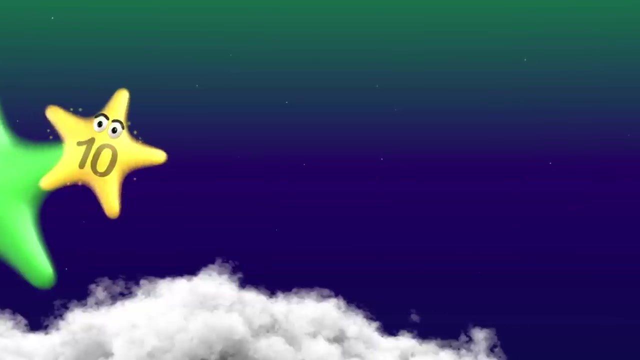 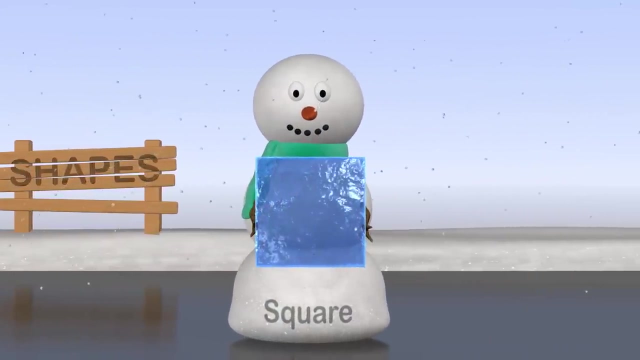 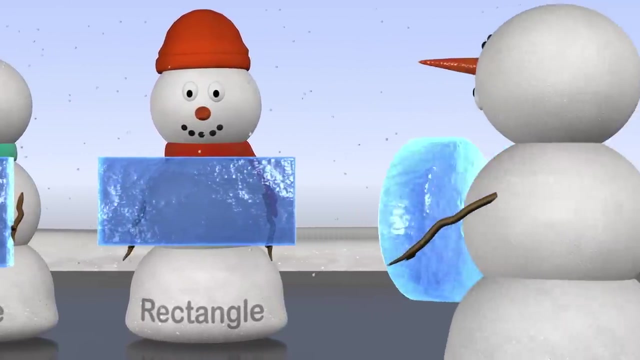 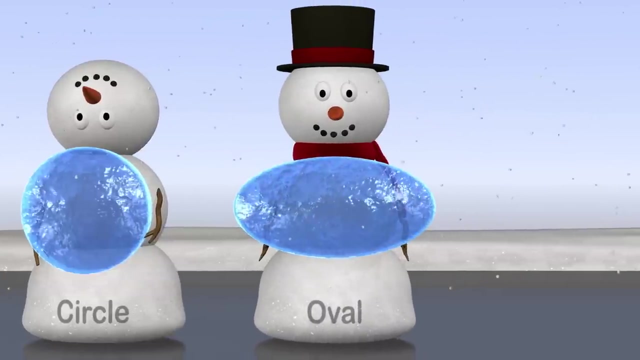 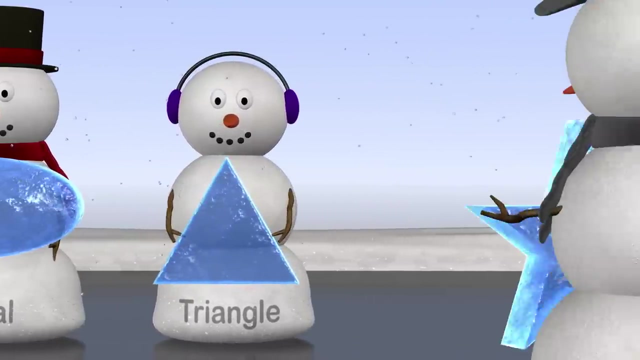 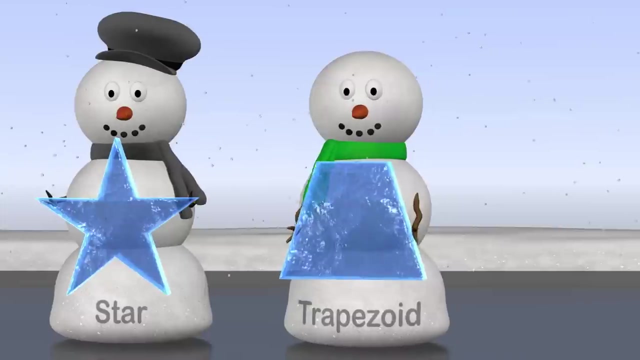 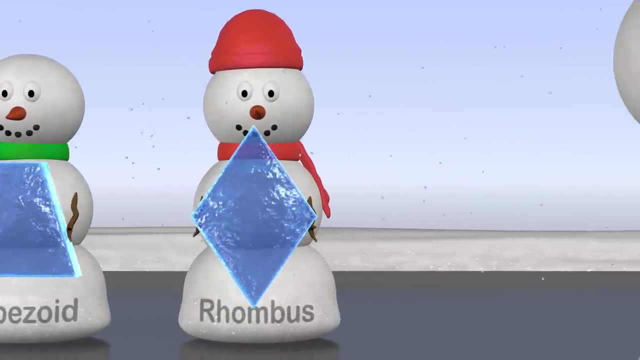 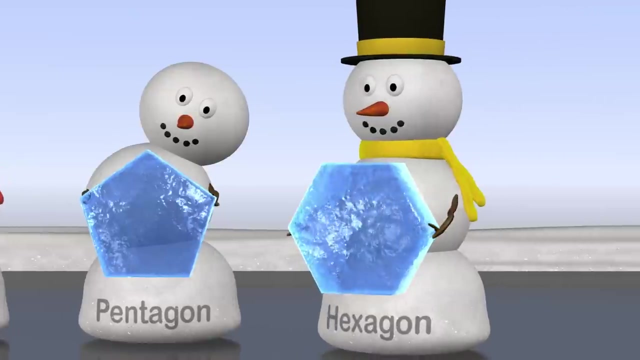 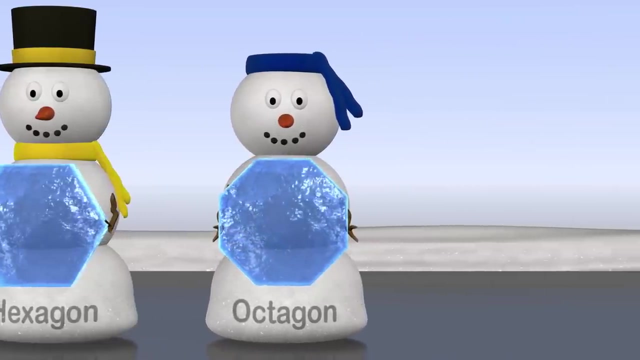 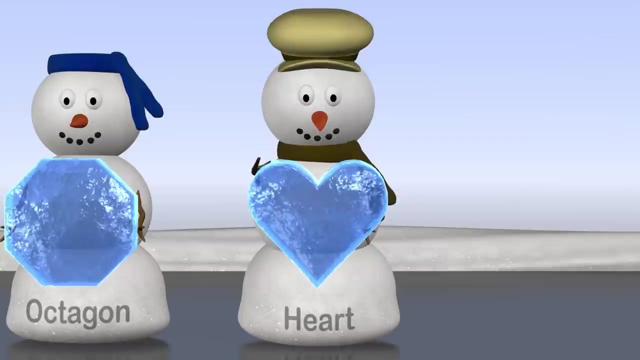 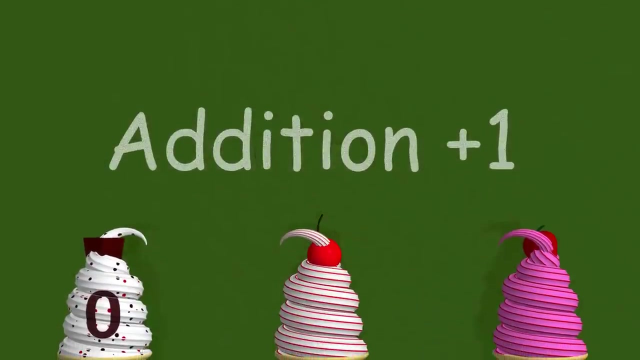 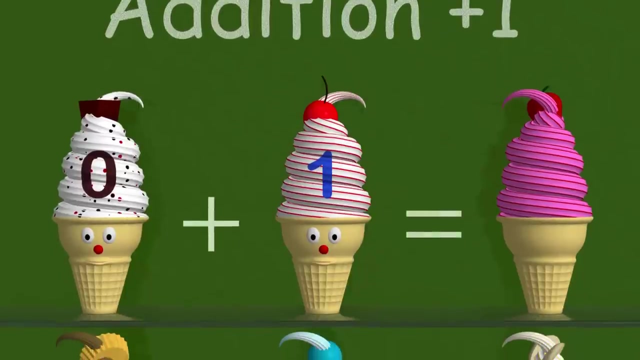 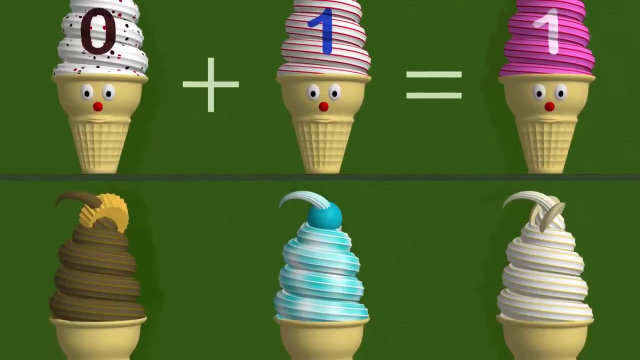 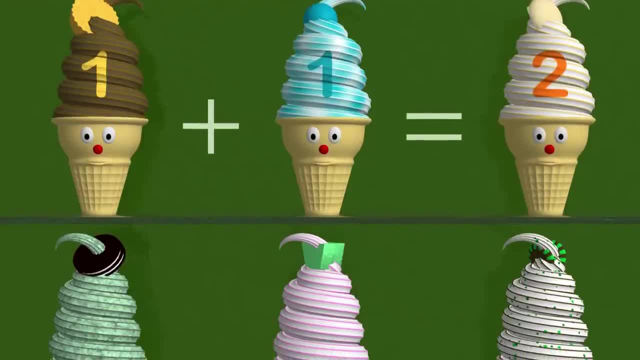 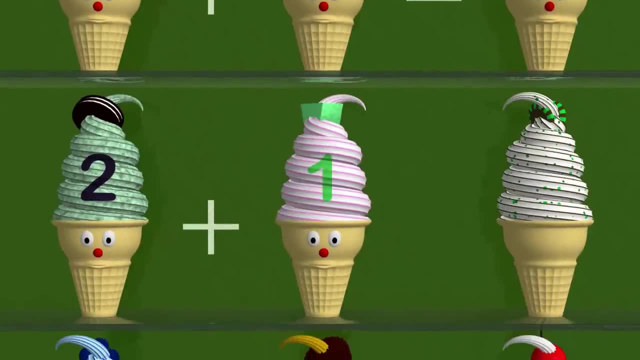 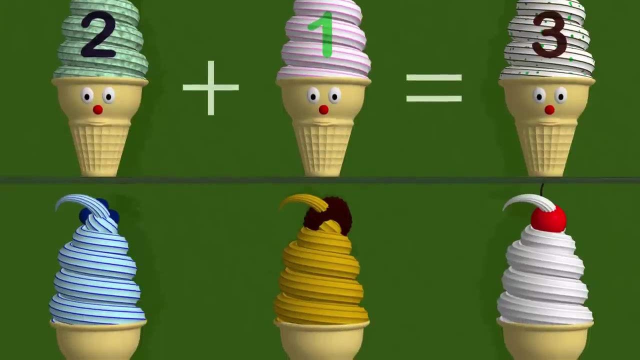 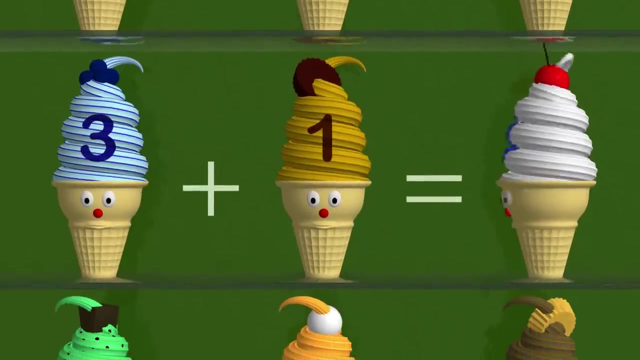 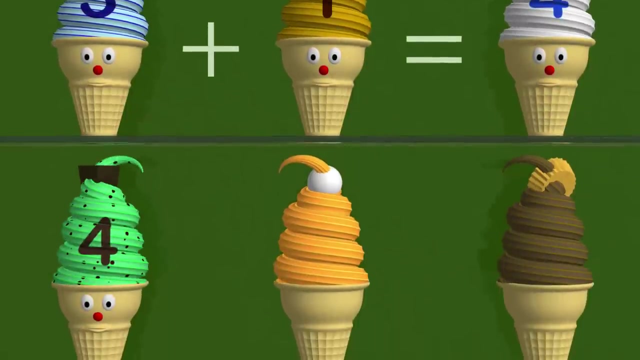 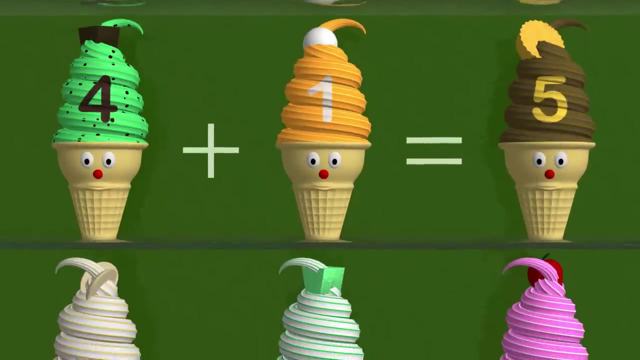 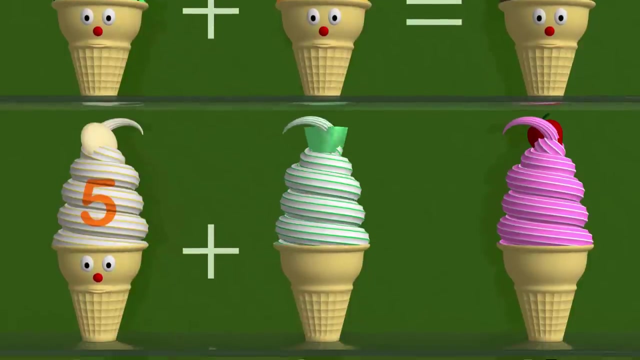 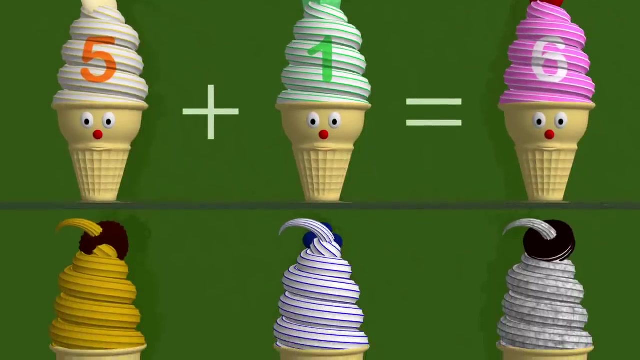 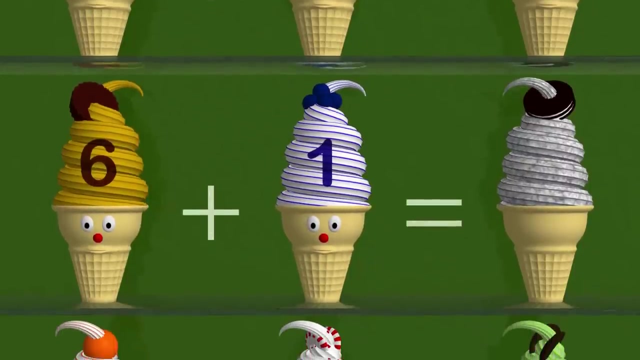 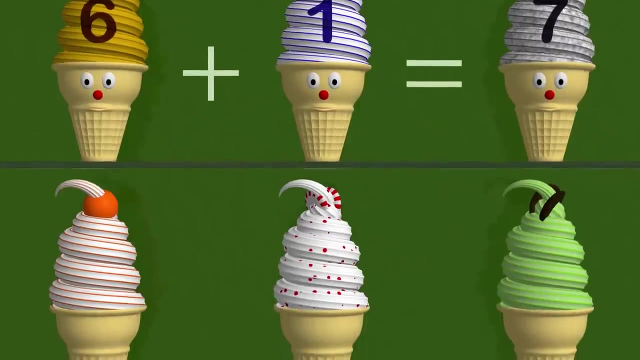 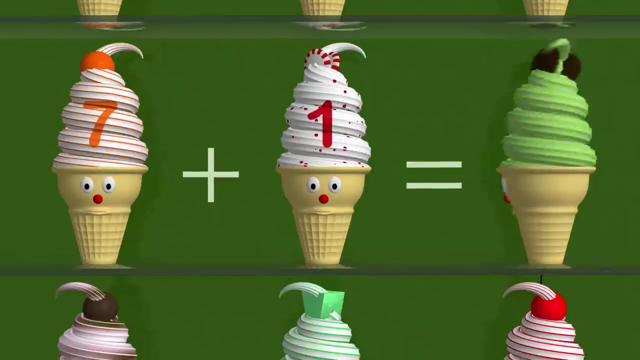 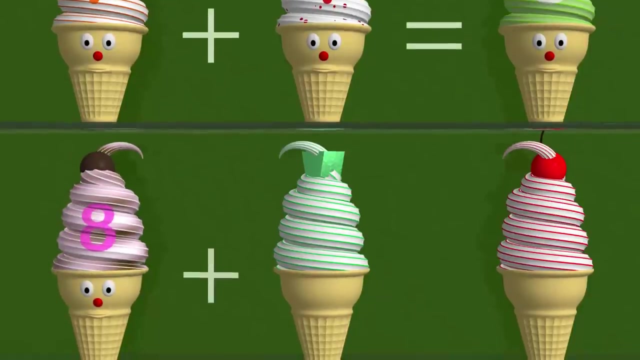 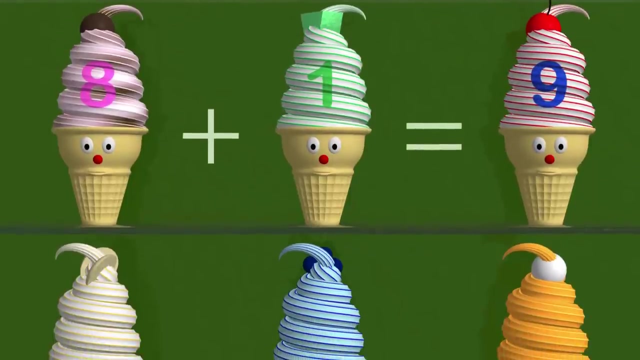 Zero Zero, Zero. Zero Zero Zero. 4 plus 1 equals 5, 5 plus 1 equals 6, 6 plus 1 equals 7, 7 plus 1 equals 8, 8 plus 1 equals 9, 9 plus 1 equals. 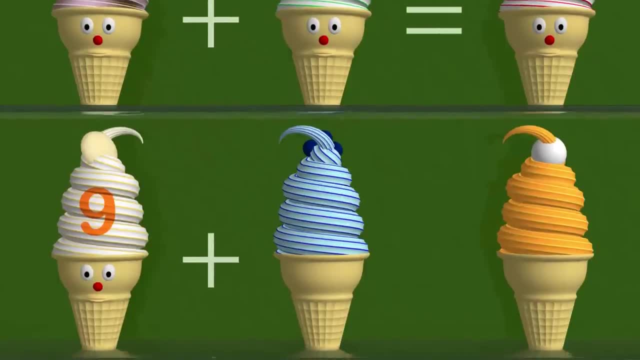 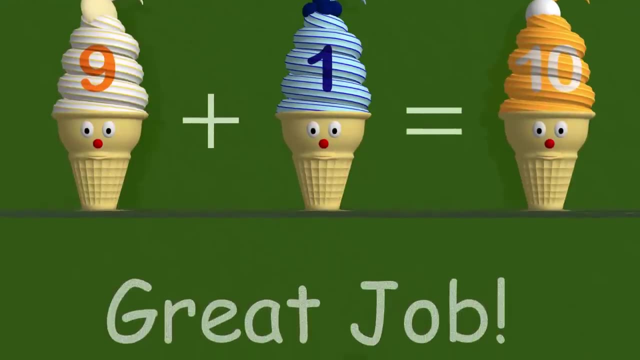 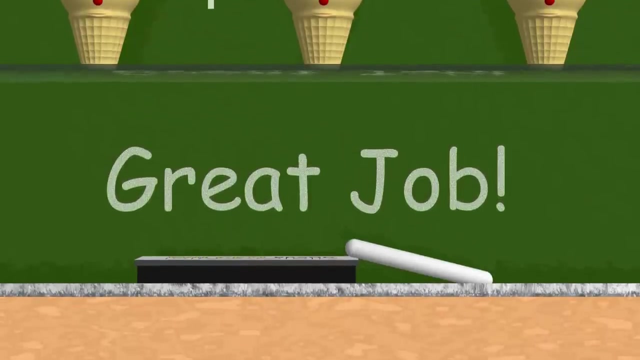 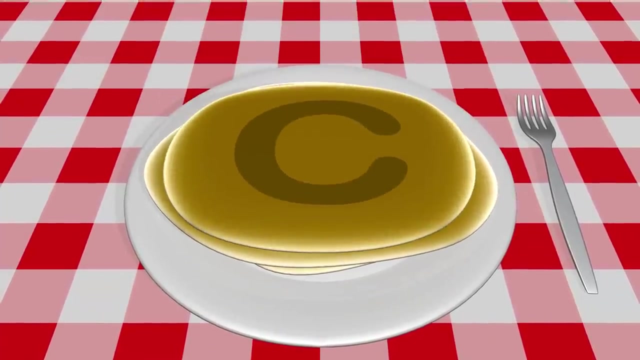 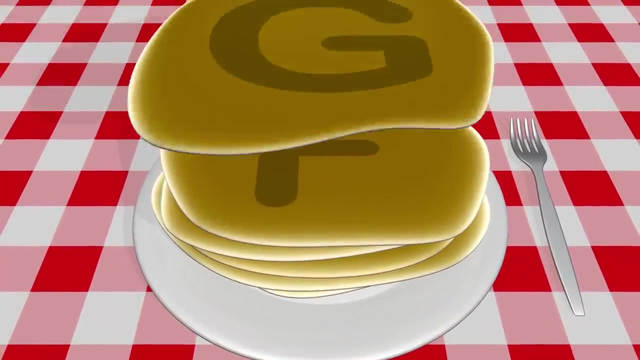 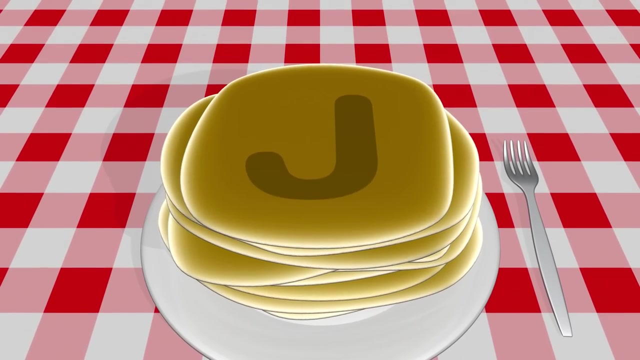 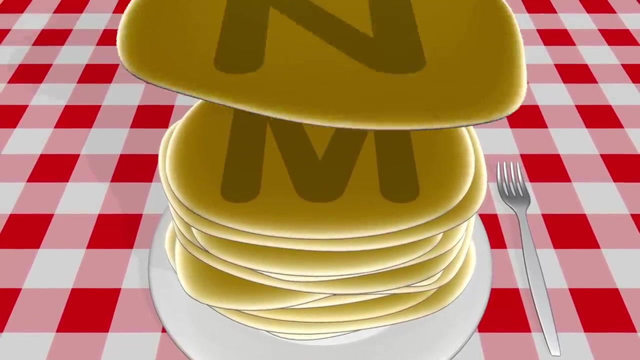 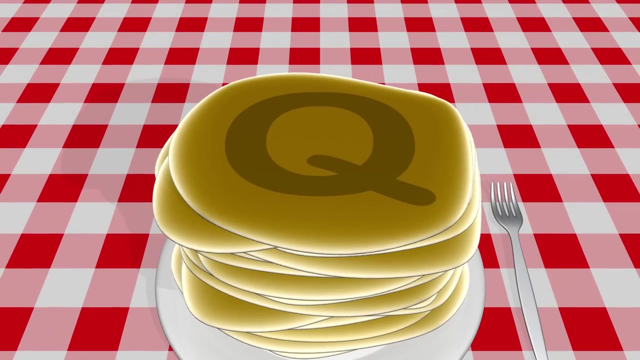 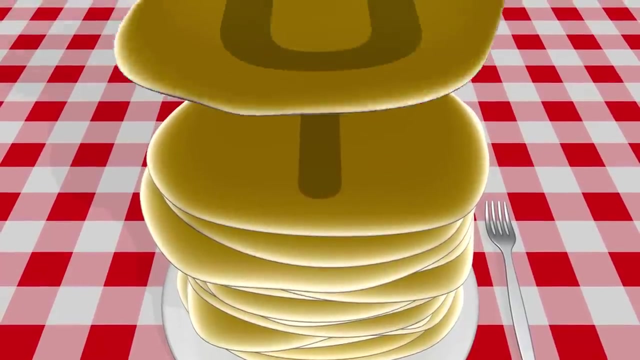 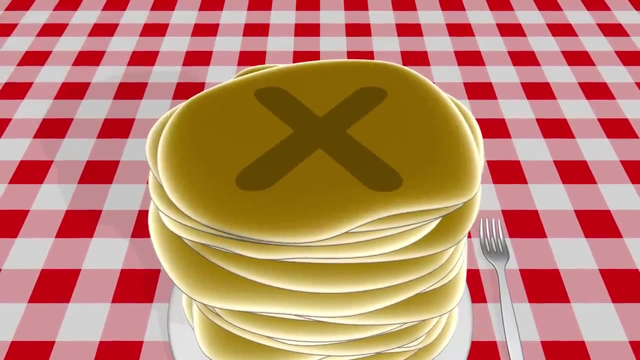 9 plus 1 equals 10.. A, B, C, D, E, F, G, H, I, J, K, L, M, N, O, P, Q, R S, T, U, V, W, X, Y Z. Thanks for watching.